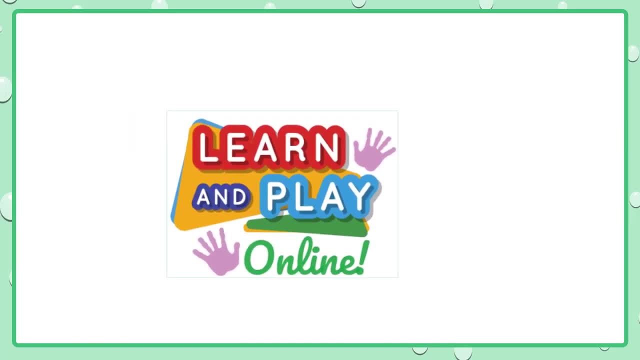 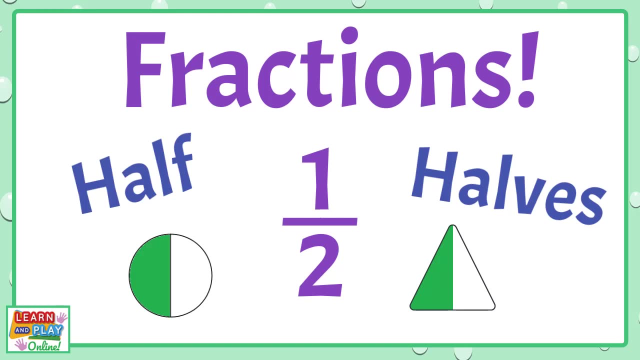 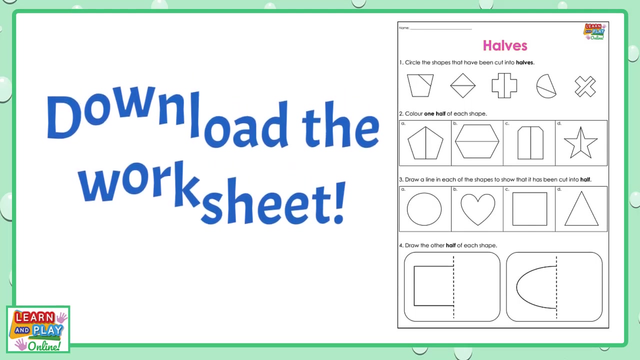 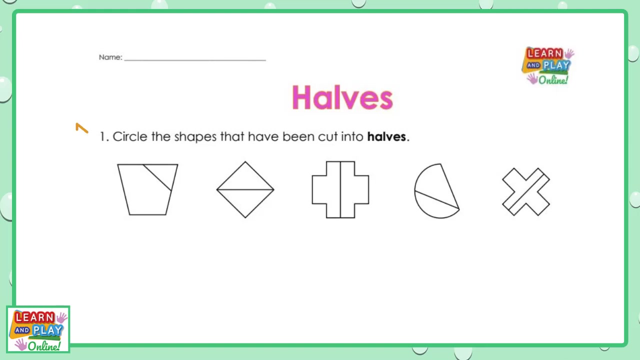 Learn and Play Online Fractions. This video is based on a worksheet. You can find the link to the worksheet in the description box. Make sure you pause the video as many times as you need. Let's have a look at question number one. The instruction says: circle the shapes that have been cut into halves. 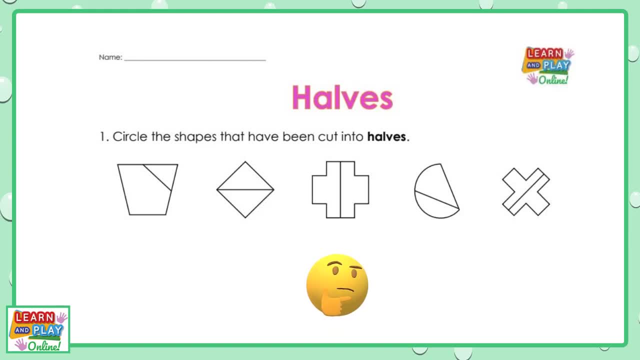 Take the time now to examine the shapes. Remember: a shape has been cut into halves if there are two equal parts. Here are the shapes that you should have circled. All of these shapes that have been circled have been cut into halves because they each show two equal parts. 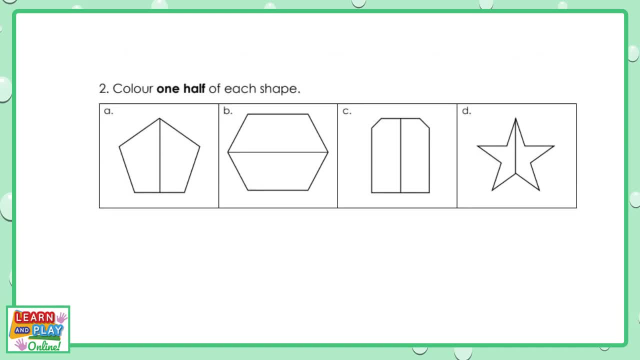 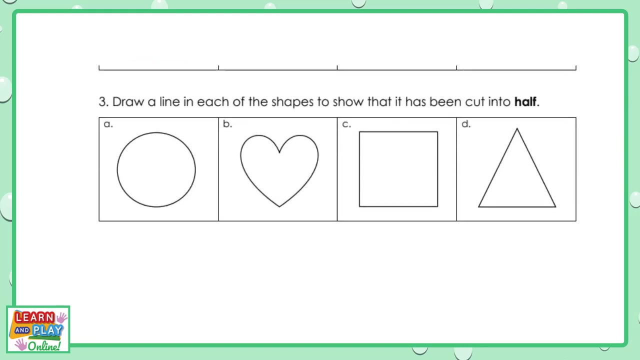 Now let's move on to question two. The instruction says: colour one half of each shape. Pause the video and take the time now to do so. Here is how you could have coloured one half of each shape. Moving on to question three, The instruction says: draw a line in each of the shapes to show that it has been cut into half. 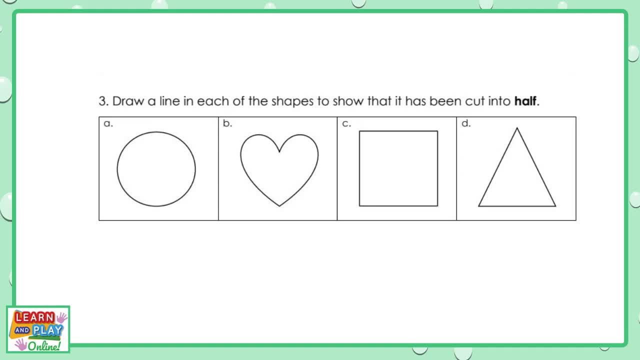 Pause the video and take the time now to do so. Remember, a shape has been cut into halves because there are two equal parts. Here is how you could have drawn your lines. The instruction says: colour one half of each shape. Pause the video and take the time now to do so. 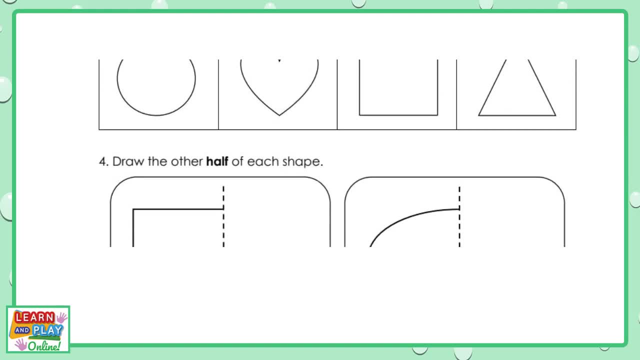 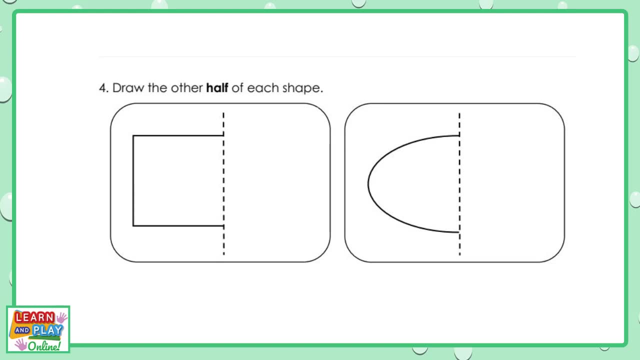 Remember a shape has been cut into halves because there are two equal parts. Pause the video and take the time now to do so. Question four says: draw the other half of each shape. Pause the video now and try your best to draw the other half of each of the shapes.